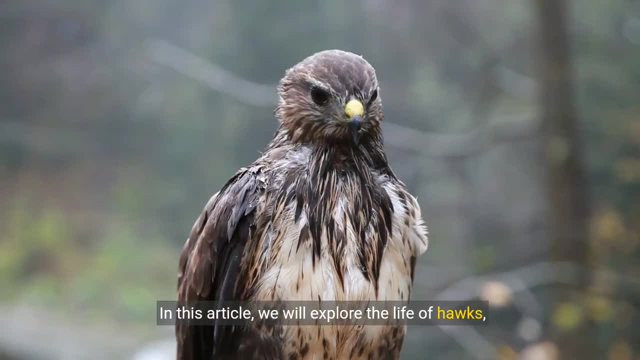 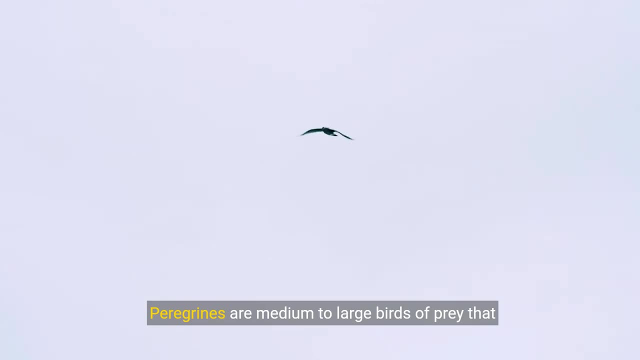 centuries. In this article, we will explore the life of hawks, their unique characteristics, their hunting behavior and their importance in natural ecosystems. Peregrines are medium to large birds of prey that are characterized by hooked beaks, large, sharp eyes and long, narrow wings that allow them to fly at high speed and maneuver. 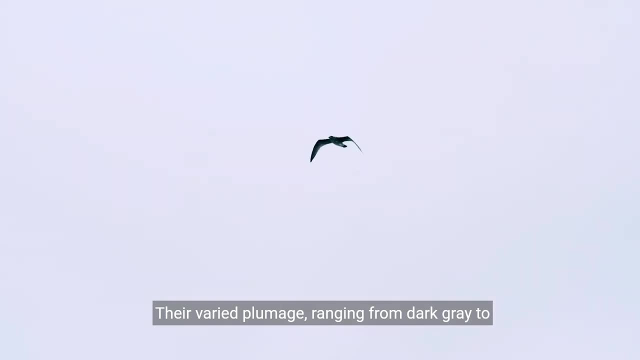 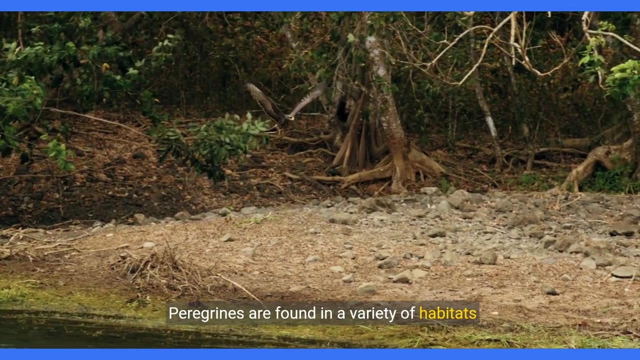 nimbly through the air. Their varied plumage, ranging from dark gray to light brown, provides them with camouflage while hunting in their natural habitat. Peregrines are found in a variety of habitats throughout the world, from forested and mountainous regions to deserts and 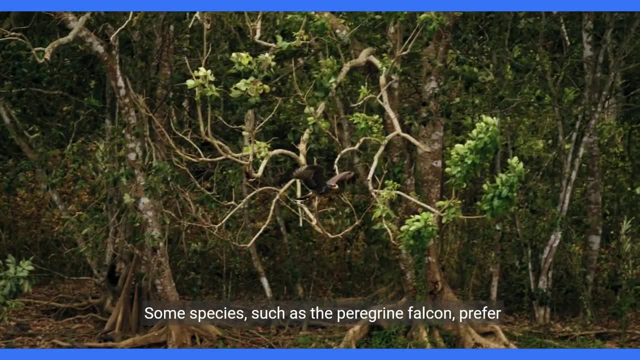 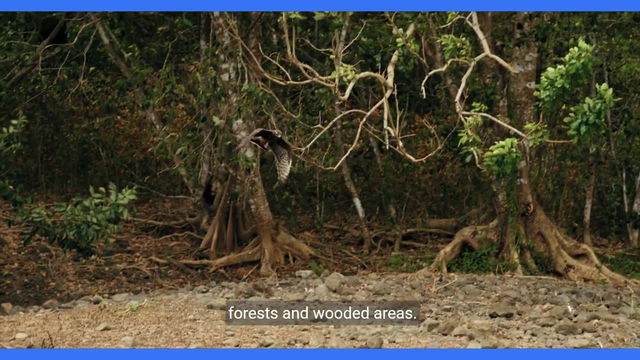 urban areas. Some species, such as the peregrine falcon, prefer open habitats such as cliffs and plains, while others, such as the Harris's hawk, are found in forests and wooded areas. Peregrines are agile predators that feed primarily on smaller birds. 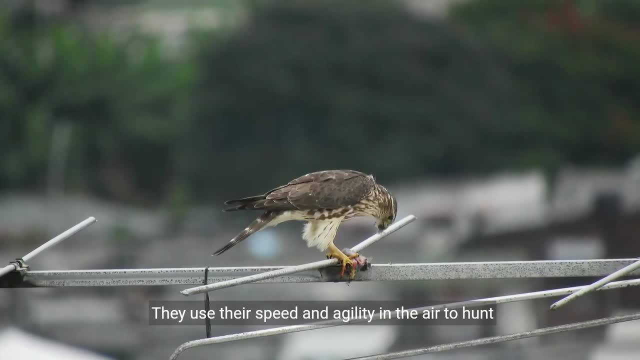 such as pigeons, songbirds and ducks. They use their speed and agility in the air to hunt prey in flight, swooping from great heights to catch prey with their sharp talons. Some species of hawks also hunt ground prey, such as rodents and insects. Breeding in hawks generally occurs during. 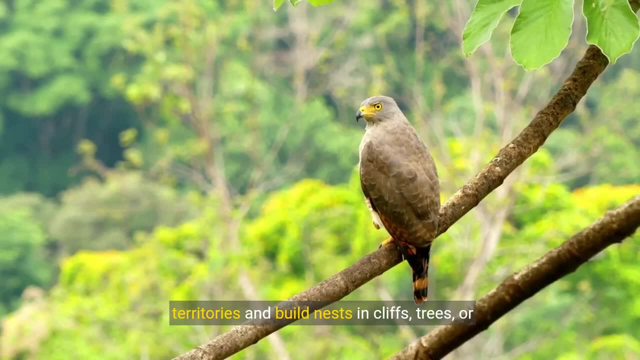 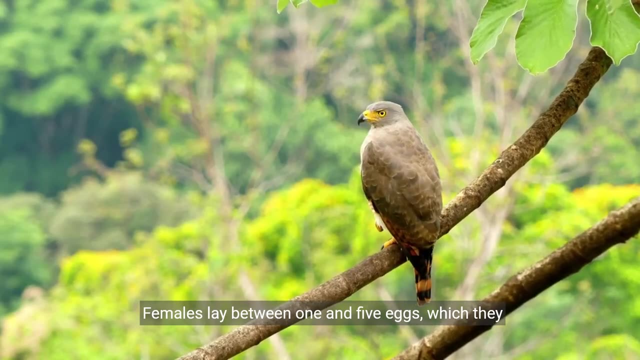 the spring and summer and in the fall, when they are able to hunt. However, they are not able to hunt in the summer, when pairs establish breeding territories and build nests in cliffs, trees or human structures. Females lay between one and five eggs, which they incubate for several weeks before. 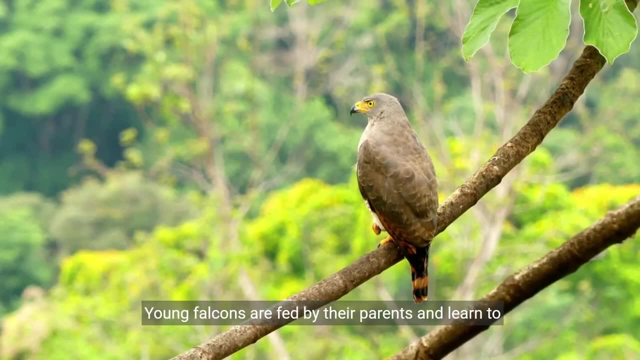 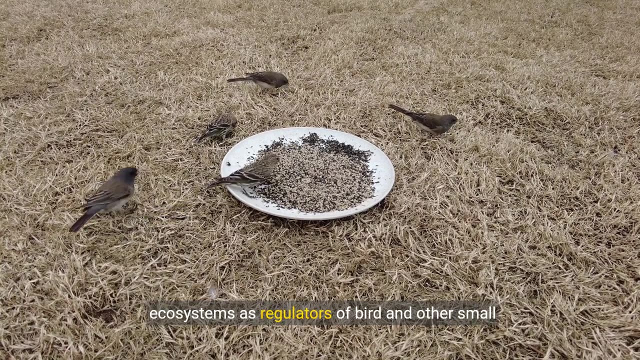 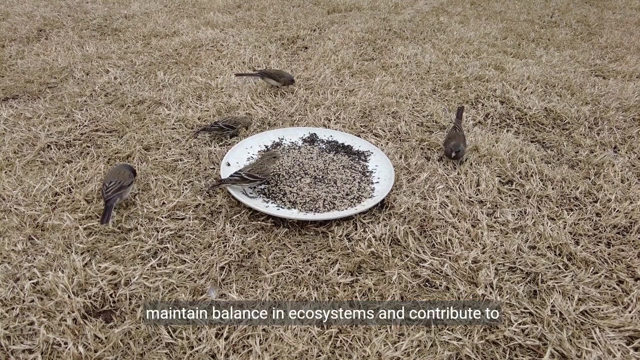 the chicks hatch. Young falcons are fed by their parents and learn to hunt and fly before becoming independent. Peregrines play an important role in natural ecosystems as regulators of bird and other small animal populations. By keeping prey populations in check, they help maintain balance. 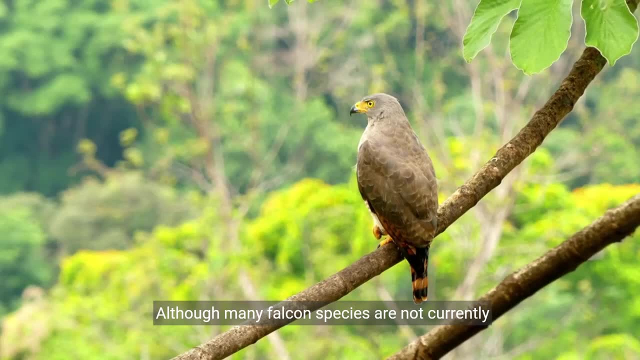 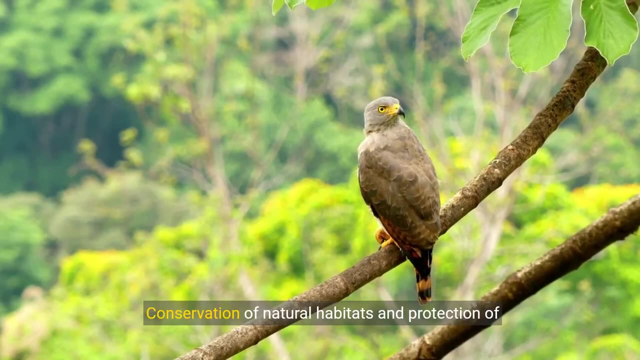 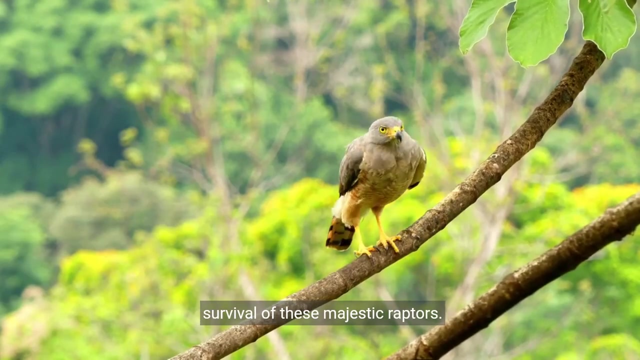 in ecosystems and contribute to biodiversity. Although many falcon species are not currently endangered, they face threats such as habitat loss, environmental pollution and poaching. Conservation of natural habitats and protection of nesting areas are crucial to ensure the long-term survival of these majestic raptors. Falcons have been hunted and trained by humans for thousands.